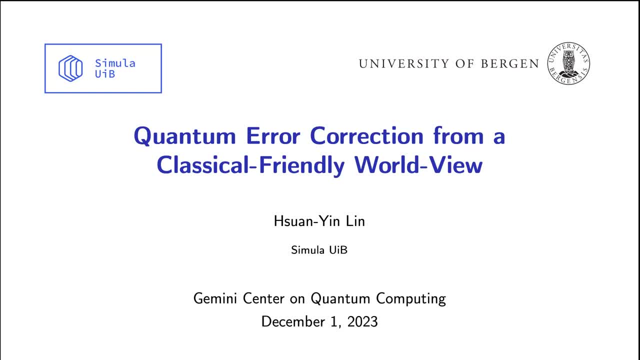 times people, when they hear about quantum or quantum computing or quantum information, they will get afraid because they don't want to deal with the hard math. So I will try here in this talk, just try to want to let you see, okay, if even we just 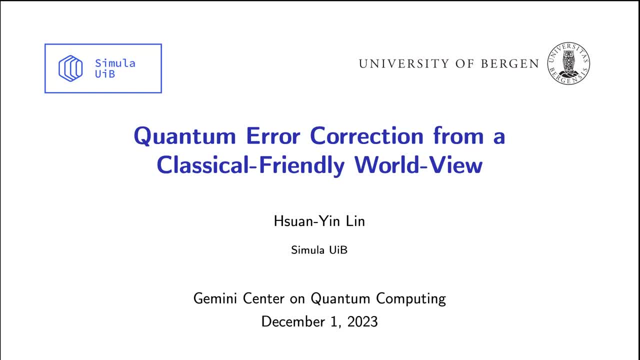 know the classical world or classical math. it's still able to understand and to solve problems in quantum error correction. But of course there's still something not happening in classical world And I will explain and how: to very small test to see how exactly quantum world would. 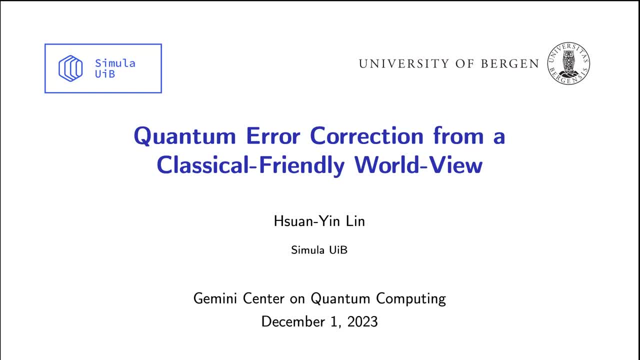 behave This kind of scenario. So yeah, I will try to make very classical friendly, But of course, if you see any questions or any problem, just Yeah, just ask me. Okay, I need to move to you, Yeah, so I mean. 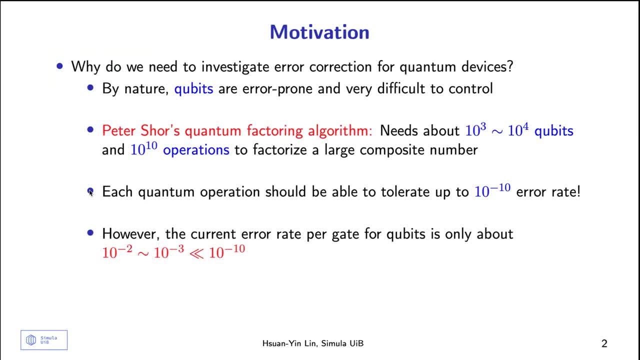 why these days quantum error correction or error correction in general? it's very important for quantum device Because the nature of the quantum bits are very unstable, So people need to describe this quantum bit by statistic or probability. So this is by nature, the qubits are very unstable. 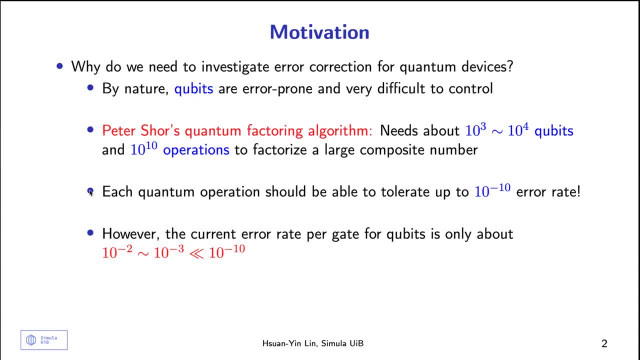 So people propose error correction to make more control, to protect this qubit, to make it more stable. And then the other hand, if you are care about the cryptography and the Peter Schultz shows that it's possible to break the quantum factorial algorithm. if you have a present computer then you can break the. 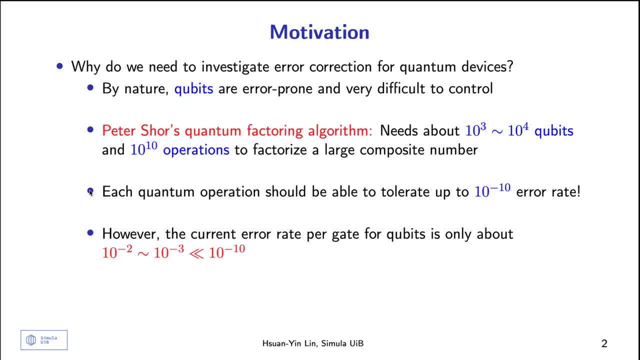 security or public key systems in the modern days. But actually it's a bit black because they need these ten to three, power to three and ten to four qubits to implement and the operations also very big for this quantum factorial augogen kum. 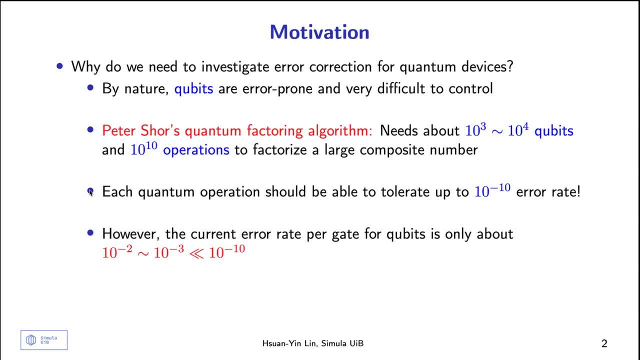 if you have heard some recent news that IBM maybe do hundreds qubits, but this is still far, far away from this kind of approach. So even you want to break this Kotaku security now, it still will not happen. That's my observation now. So 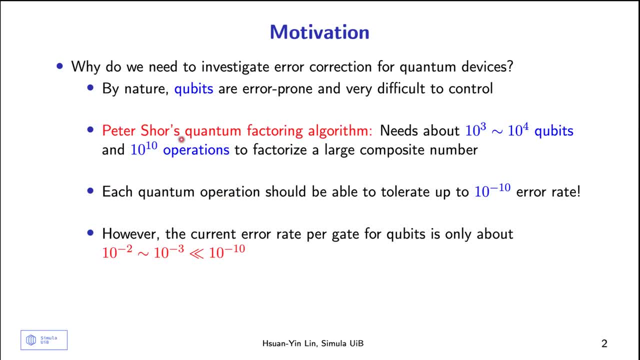 but anyway, so we can conclude that. So we need at least need to tolerate up 10 to a minus 10 error rate for implement these 10 to power operations. Otherwise just go to something errors, which is also you cannot get correct message. 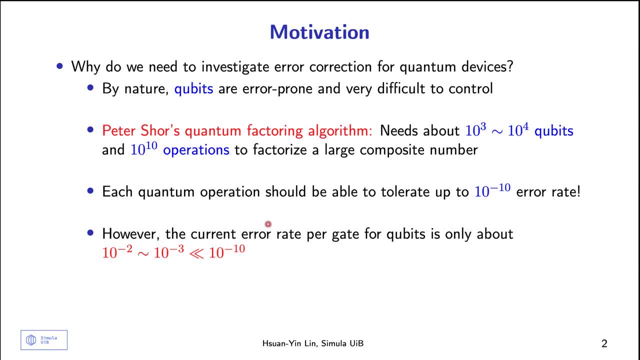 So the modern state is in general. I mean, of course these numbers actually keep updating in these days if you have keep track on the content, magazine stuff- But in general it's just 10 to power MS2 and 10 to minus 3.. 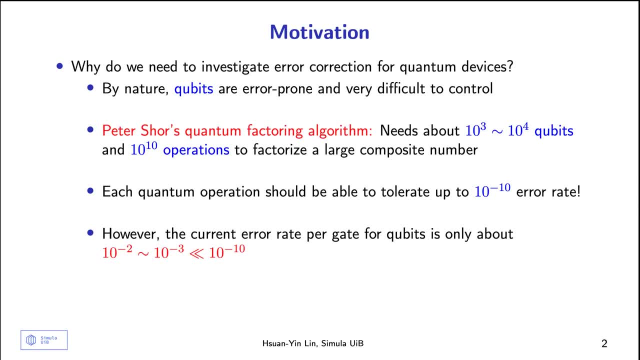 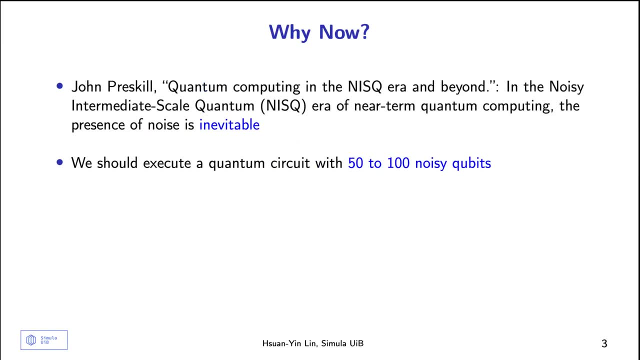 So again, this is far away. we can do So, but to me for research, to me for information during coding, I mean to me why it's actually for us to do this right. So the, I think it's like a father of. 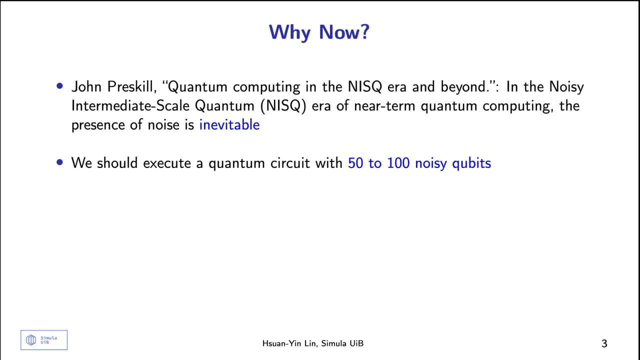 quantum computing Preskill. But anyway, he predicts that I mean in at least 20 years, 20 years or 30 years. I mean you will not avoid the quantum noise, the qubit noise, in this time. So no matter how quantum device you design, 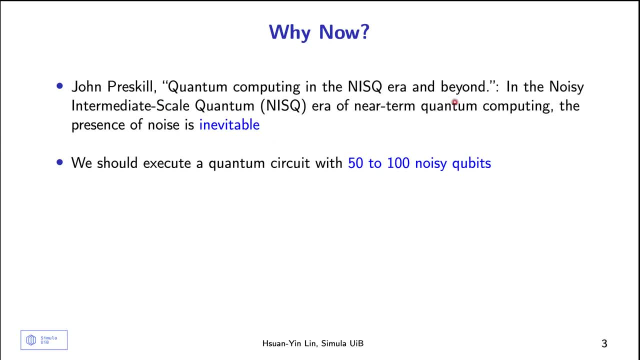 you will always match the noise. And then if we want to implement some quantum circuit in practice in hardware time, then you will need, of course- I mean you will encounter- 50 to 100 noise qubits. So this is for sure. 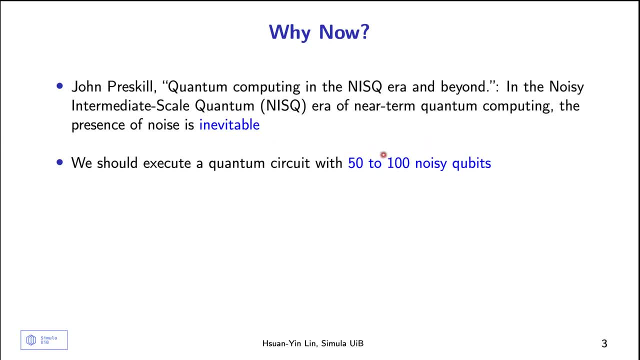 So this is actually quite a small number, I mean compared to the telecommunications in classical. But to me I think it's the right time to do that because if you have observed the quantum- sorry classical information theory actually in these times, 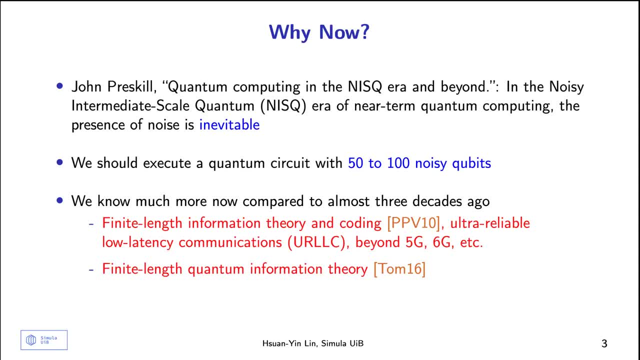 these three decades, 30 years. so people actually also work on this. very practical. the problem is okay. the code is called finite length information theory, So they just care about small number of bits and how much information or message you can transmit. 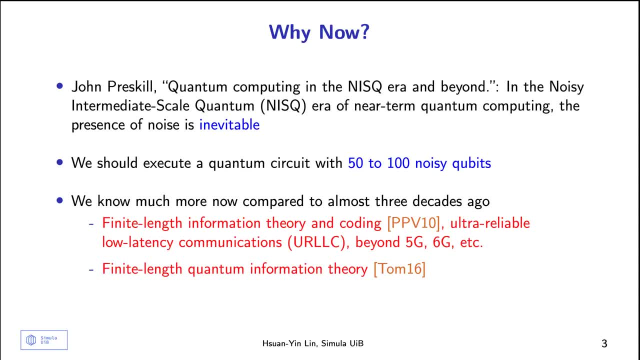 And then also how the coding can do with these small number of bits. what's the best and what are the fundamental things. And these things actually also not just happen in the classical world, So in the quantum world there's also. people study finite length. 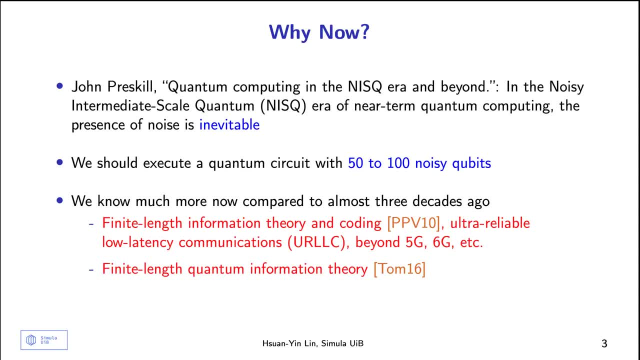 quantum information theory. So the benefit for us now is that actually we can use all these tools developed in 30 years such that we can make sure: okay, what's the best we can do, even we have 50 to 100 noise qubits? 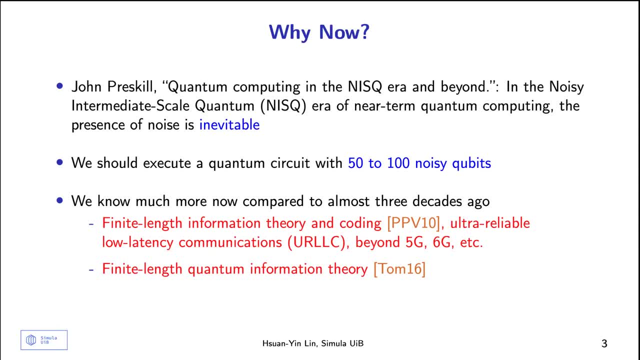 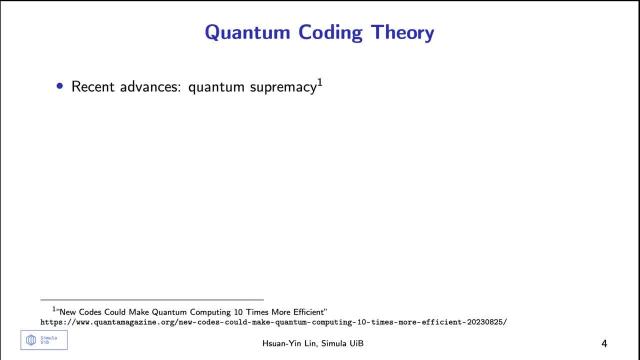 So this is at least my motivation to do this research starting from now. So just talk about very general, how quantum coding theory actually is used in I mean this year or last year. So of course, there, you all know this supermercy keyword. 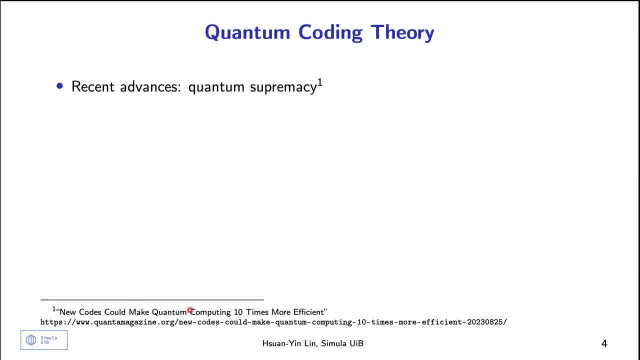 but in recently there's some researchers- you can see this magazine- So they showed that, okay, if you've designed a very good quantum code which is stabilized code- I will talk in this talk- that you can actually make 10 times more efficient. 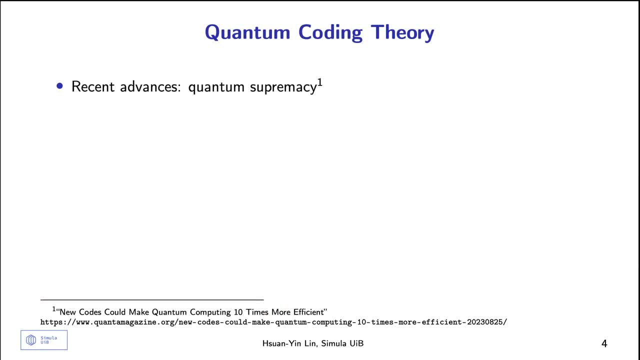 than what they currently have. So coding actually helps a lot in building up these efficient quantum computings. And these are also, I mean, technical names, but just to let you know, the modern good quantum code, some surface code or color code. 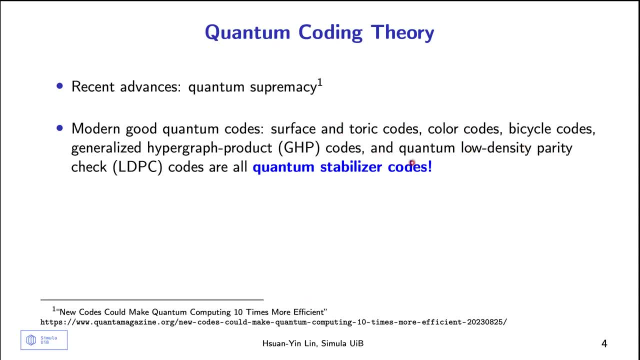 bicycle code- this fancy name- and also even the most popular codes in this year, I would say, is quantum LDPC codes. They are all actually quantized by stabilizer codes. So in this talk I just want to give you a tutorial. 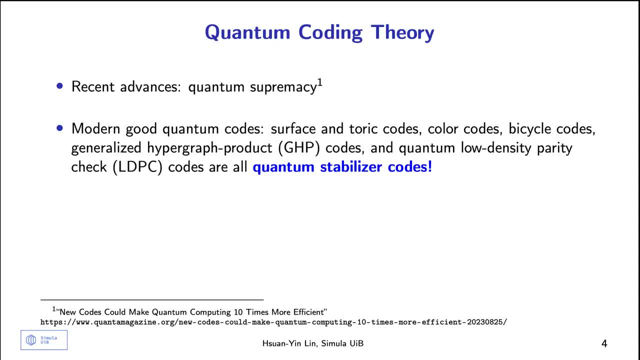 on how, actually why it's quantum stabilizer codes, Such that actually we can understand okay why this can do. So just a brief story: So the 10 times more efficient is that? okay, people, they can find quantum LDPC codes. 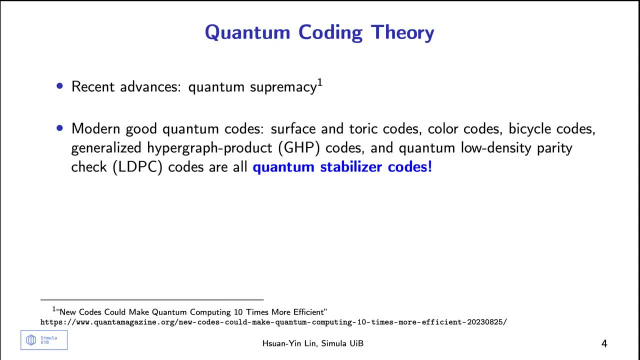 which is very efficient. in classical LDPC code It's better, much, much better than 10 times more, better than this code, surface code. So surface code was the previous popular code, but now it's beaten by. I mean, but of course these are just simulation. 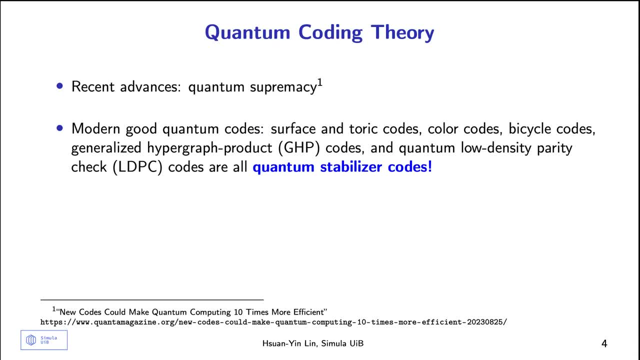 It's not talking about hardware stuff still. So this is just a prediction, but still, if you talk about hardware and circuits, there are still a lot of things to to to discuss so recently. why it's so public, because there's a famous computer science conference, doc uh 20 2022. so they actually have two papers, got a word and 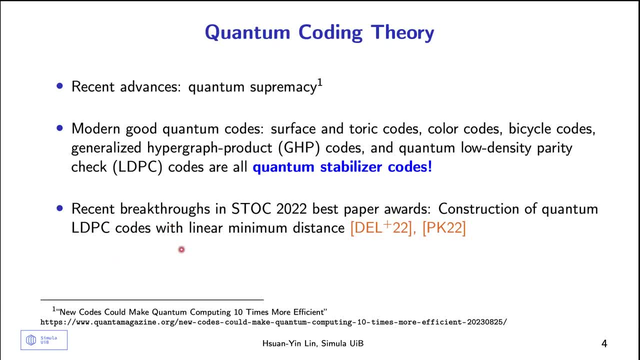 they all talk about quantum ldpc codes and they show that the the the minimal distance of such code grows linearly in the qubits, which is- uh, they believe, is a good call, because in classical i think a lot of people can even do almost better than linear. yeah, so they want to show some. 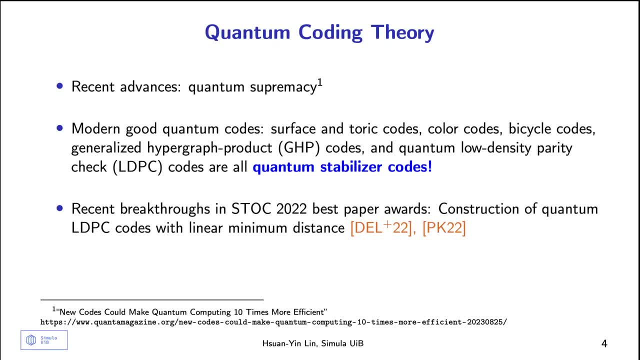 similar, similar property in quantum version, but- and this actually is an open problem- i think 20 or 30 years or so. but i will talk later, once i start to explain the code. so maybe you will know why it's actually so hard to to find such good codes with the linear minimal distance. 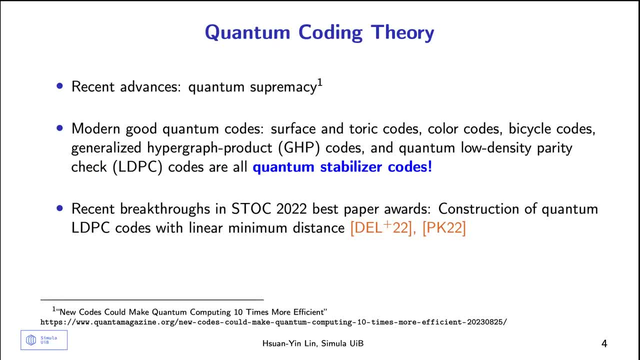 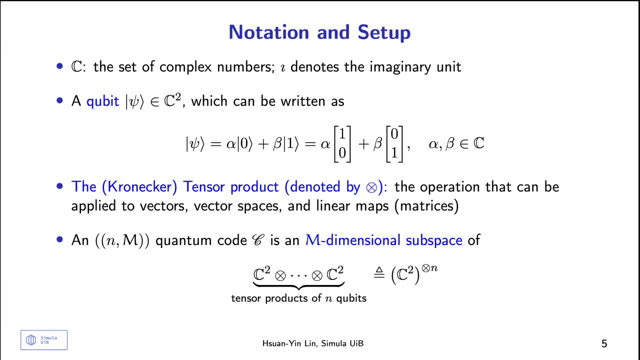 so, uh, okay, so this is my motivational story, so let's just go to a bit boring part. so i mean, it still cannot avoid. if you want to know quantum, you still need some math. but the most math you need actually just not just but linear algebra in classical you also need this- and then the most, i think, the knowledge. 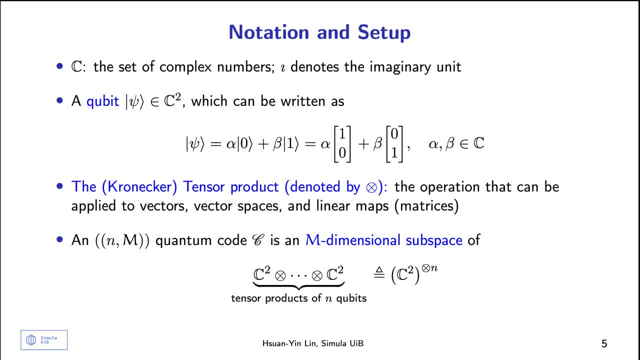 you need more is actually they call matrix analysis. so matrix analysis is much more different from what we know in a classical world. so i will just introduce notation first. so this is a complex number and this is the, the imaginary unit, and what we call or how we. 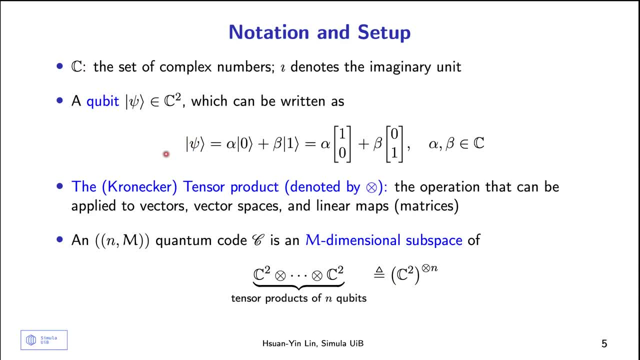 call it. now is政府 in classical use the curve function and then we have a computer, and then we have the computer, and then the computer and then the cube. it is just, we just use this notation. they call this the rock notation. brought in cat and they didn't do no. 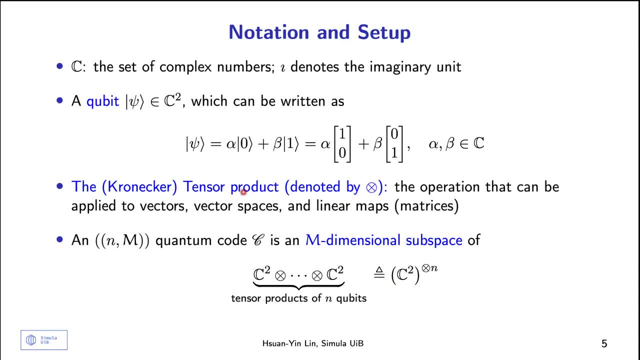 least like. so one zero and zero one. you can think about like two bases of the complex field and the alpha beta, just some coefficients of all the qubits, and then you can still get classical discretion. So now go to the point. So what do we mean? a quantum code. 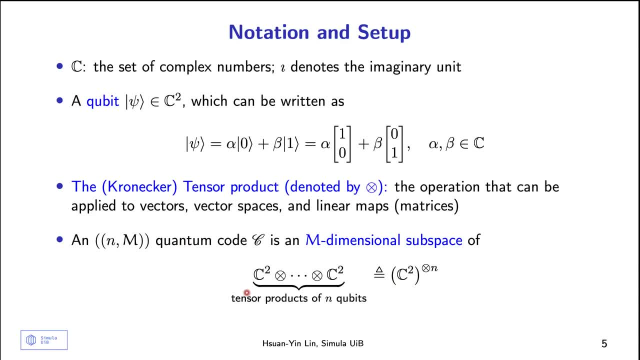 So we want to define a code over the space, of this space And the, such that this code has N capital N. you can think we call it N dimensional, but you can think about there's a capital N, the linearly independent vectors in this field. 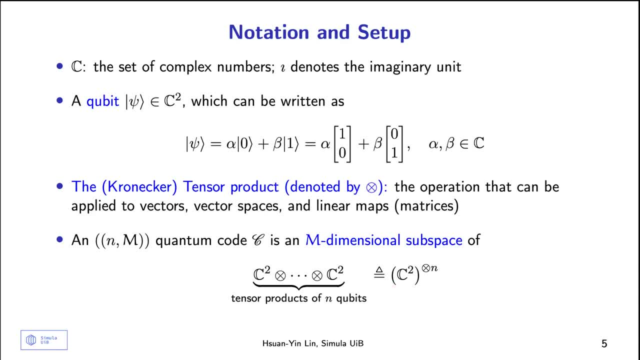 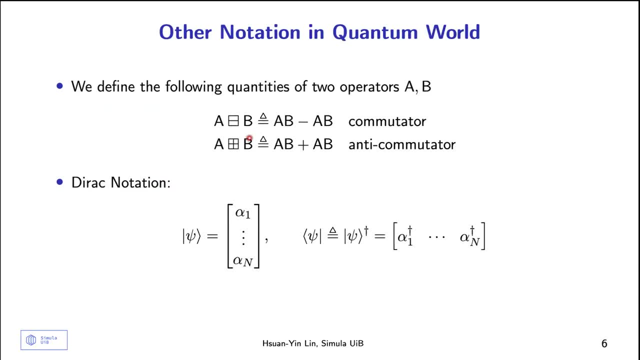 So these are just. you can think about the linear algebra, So I just use the other notation because that will be used later. So in the matrix world, so matrix analysis world, you need to also define something called commutator, So, which means that you need to simplify this. 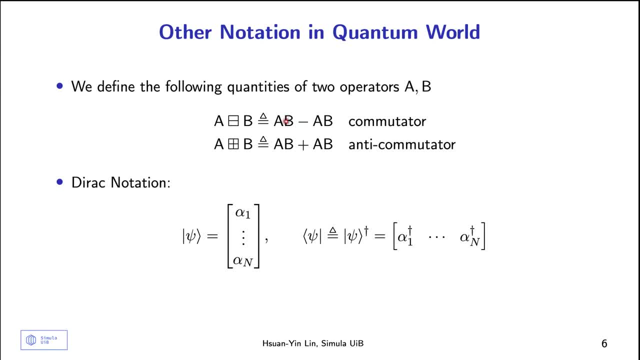 AB minus AB. Yeah, sorry, I didn't know the typo, So it should be AB minus BA, And this is as well. so AB plus BA. Yeah, so this is typo. yeah, And for direct notation, just to let you know. 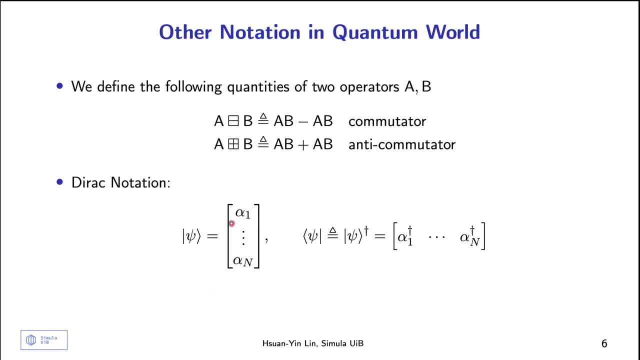 it's that we use this as a column vector. This is ket and this is called bra. Bra is just a transpose conjugate, So you can write down the vector like this: Yes, So this is also yeah, you can write it. 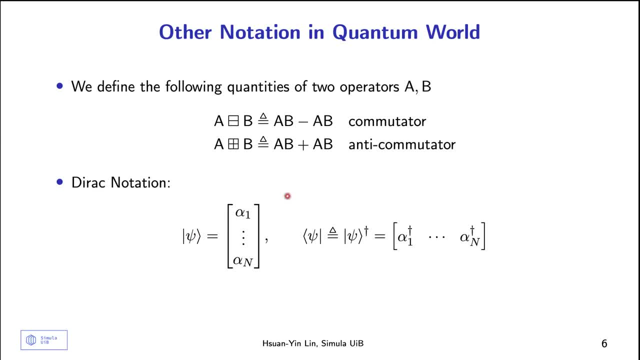 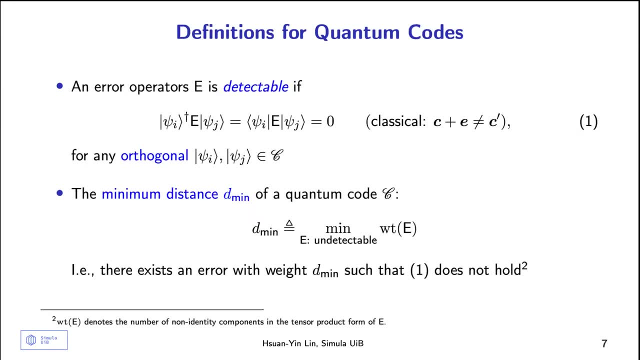 It just the notation was. maybe you are not so familiar, but if you think everything like a vector and the matrix, then it's easier. So now let's go to the general part. How, what do we mean? quantum error correction, right. 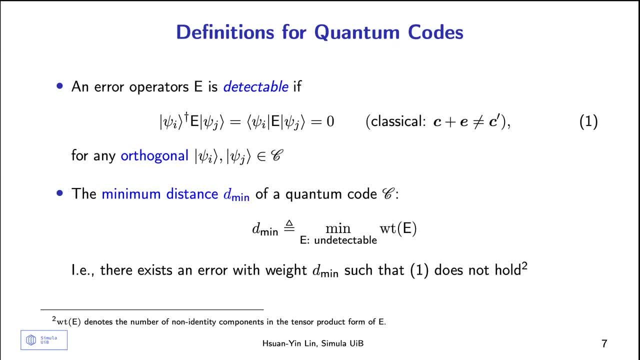 So because we have the basis right, So because we have the basis right, So because we have the basis right, This is for the quantum code right. So n kept n linear, independent code words or vectors. You can think of it this way. 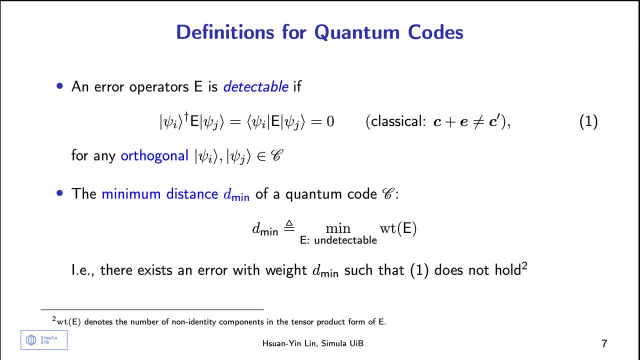 But in quantum world all the operations actually made in the multiplications and they are made by the operators They call operators. actually it's just a matrix. So it's just a matrix and operators working on this And a call is called detectable. 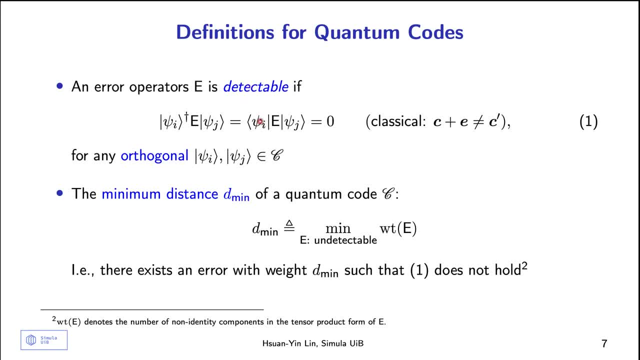 because in classical we also have this property, So it's called detectable if we pick two orthogonal basis and certify this. And again, maybe it's very hard for you to think about why we have this, but we can think about classically. 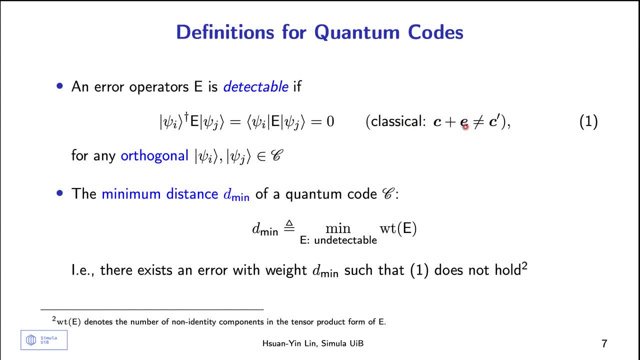 What do we mean in classical? An error is detectable, right? It's actually quite easy, just if you have a set of code words but you find an error and then you make this error. actually, it's not the other code word. 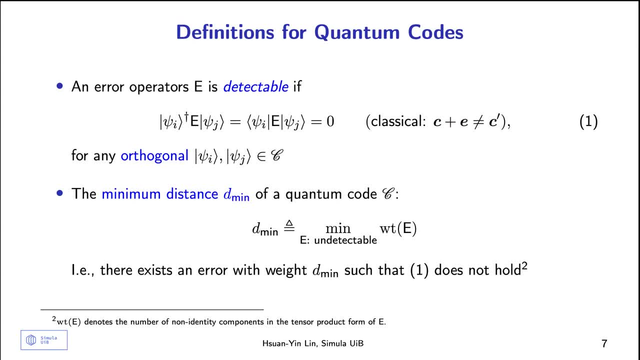 then it's detectable because it's not in the set of your code book. So this is the same right. So you have error and then you try to find the other two code words and then you cannot guarantee zero. then it's undetectable, yeah. 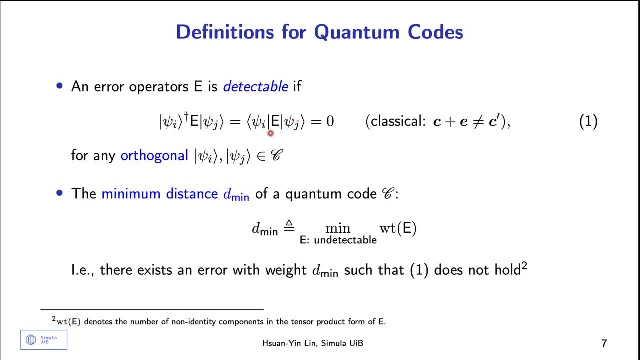 So this is just the classical. of course they have a lot of quantum theoretical discussion why this works, but this is a easy way you can look at it from a classical way, And so the minimal distance is also similar to, if you think about classical right. 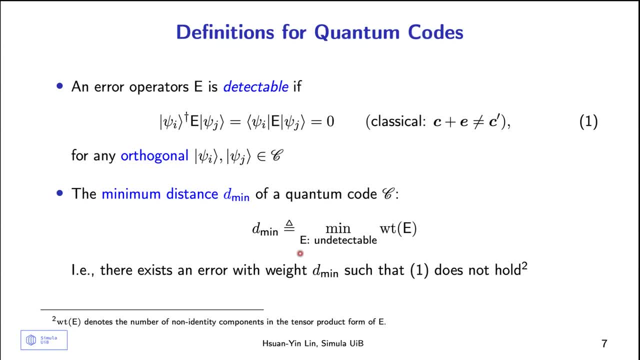 The minimal distance is the minimal undetectable error, errors among all the error operators. So if you think about the classical world, right, You have two code words and the undetectable error is the distance between these two code words. So they define the minimum of all those of them. 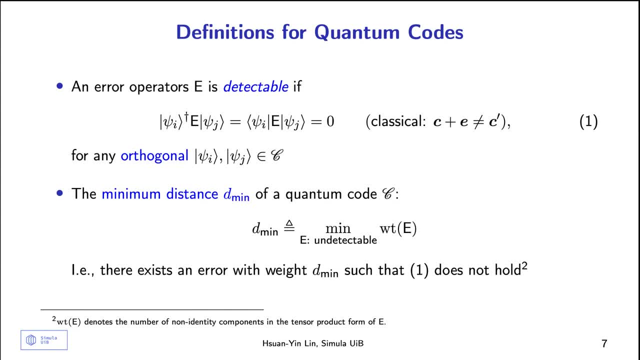 Then this is the minimal distance in quantum, same as the classical world. It just you need to think about multiplication and then think about addition. yeah, And the least definition is just some number of the matrix and which is non-identity components. 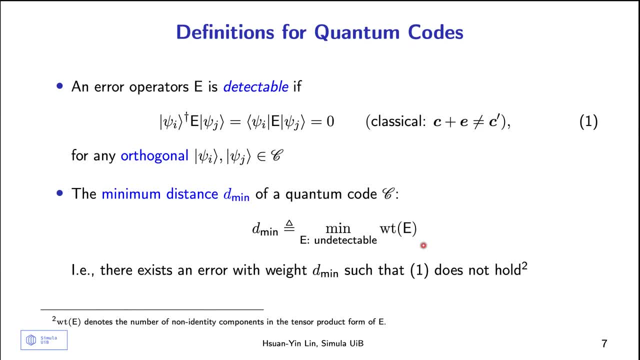 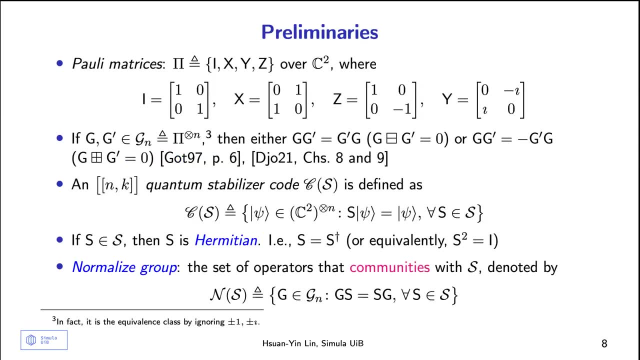 And maybe not clear here, but I will talk more clear later. Yes, So again, in classical we can describe a code book by the field size or field Right, The finite field, if you are familiar with Gallois field. 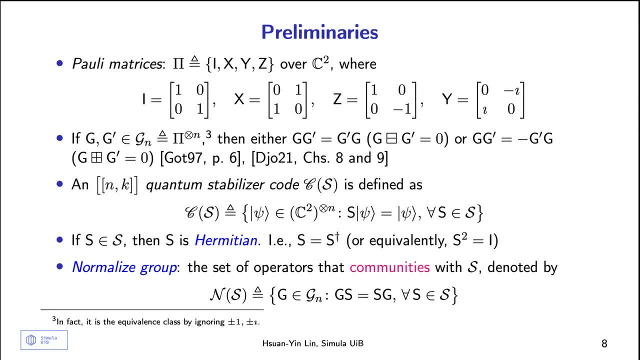 so is GFQ. So in quantum actually we can do similar. So we define something they call Pauli matrix and you have I, X, Y, Z and you can think about. these are the finite field elements in quantum world. 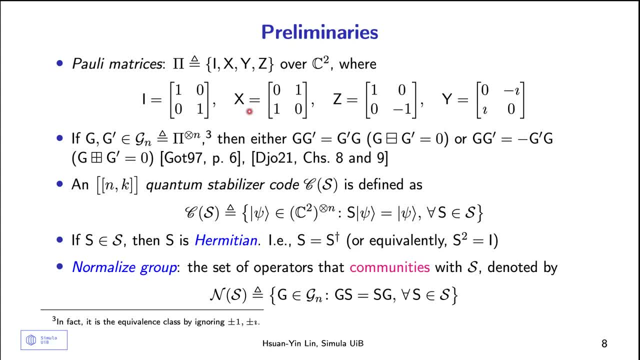 just these four, And then so you can think about a way that you think about a space, a complex space in n-cubics is just a multiply, a tensor product of these four. Right, so you can think about, it's a Galois field size four, and then it's tend to be n-cubics. same idea. 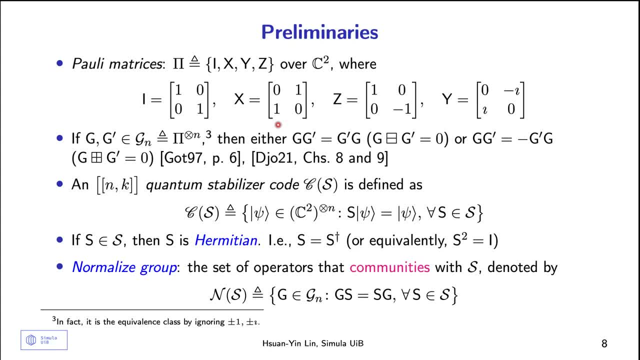 But it's not just that actually. so people actually can show that, okay, if you just work on this Pauli matrix- they call this Pauli basis- it must satisfy these two conditions: First, it communicates and the other is anti-communicates. 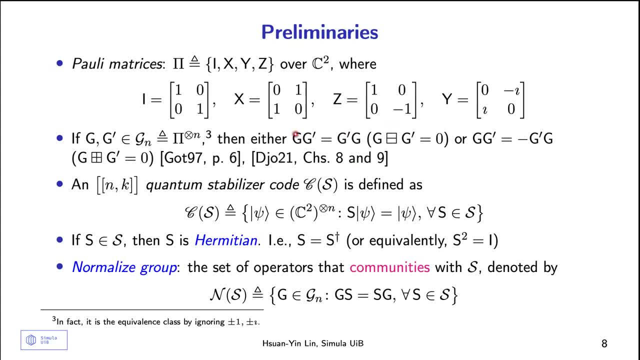 So this must be satisfied in these things. And the one thing I didn't specify by the math is because this is a bit complicated about quotient stuff, So here It's kind of it's called equivalent class, So it's not just all the Gn but just the equivalent class of this Pauli matrix. 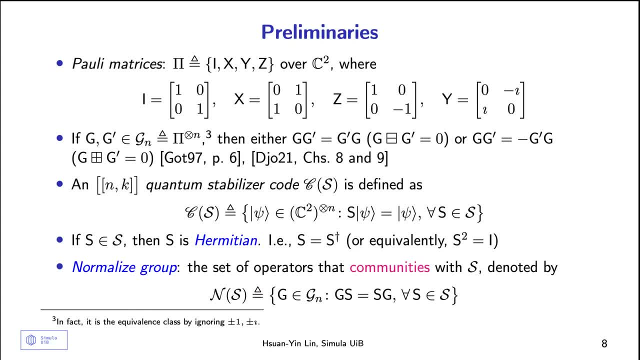 But I will not talk too much about that. So now we can go to the main topic we have today. It's the quantum stabilizer code, So it's defined by this. So you want to find a code or vector basis in the complex world. 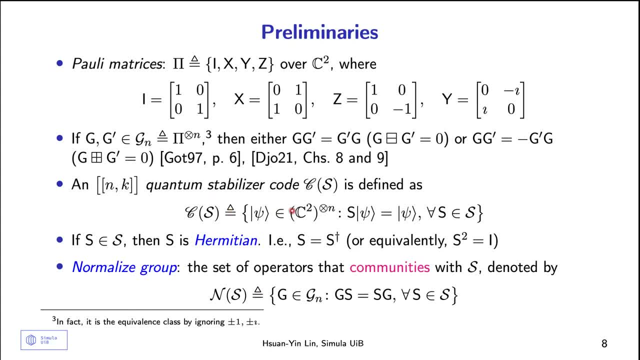 And the least base is defined by: okay, you pick some matrix, actually it's m minus k matrix- and then you ties the vectors. it's still back to the vector, which means it's the eigenvalue one space. So it's again also linear algebra, eigenspace one. 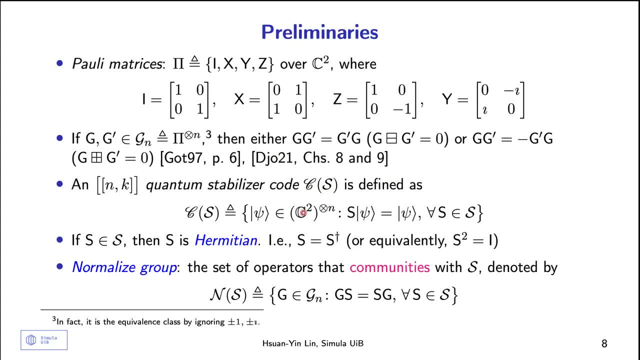 And then they use this to be as a quantum stabilizer code And then they actually some history reason why they define it. So the most, I think, intuition for me is that why they need to define it, because in quantum world the most difficulty to do is that you still, because you want to send some information in the quantum world, right, 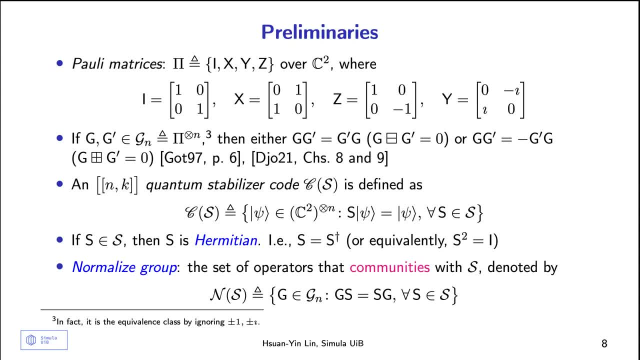 But still, we are living in a classical world. we want to attract this kind of information back to classical, And then we need to do a measurement, like physical measurement, right? So we need some very- I mean- fancy device to measure. okay, what's the state of this information? 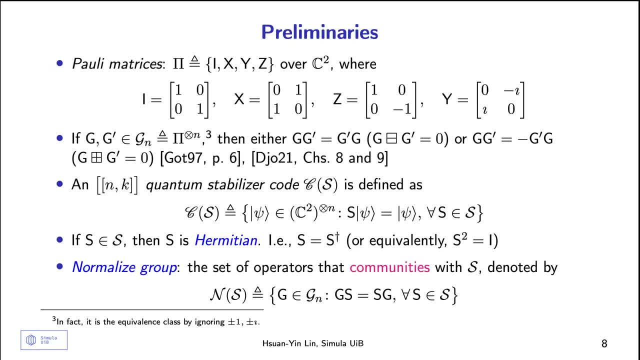 What's the other state of the other information? So these stabilizers can be thinking about like measurements. So you have a quantum code exists by your construct, but you do some measurements such that you can explain the mathematical phenomenon. So this is the intuition. 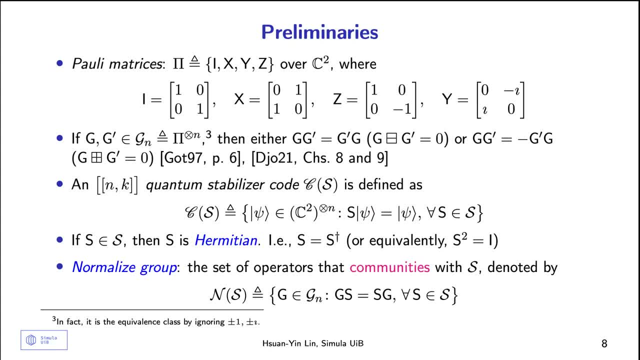 The why this stabilizer code can think of Yes, And then, of course, based on this definition, people can prove further, which is actually very useful for us for error correction. So, for example, this must be a Hermitian. 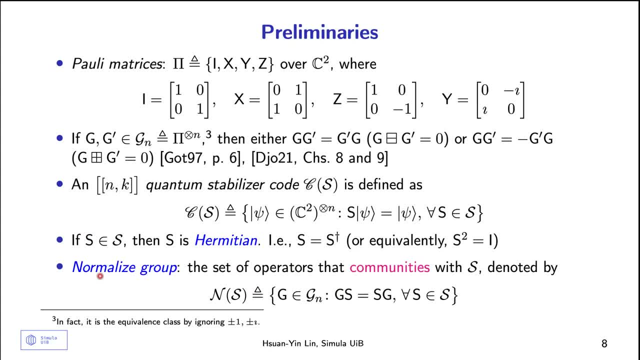 And if you know something like algebra, they would also define something called a normalizer group And it just you pick, because this property right, Because either it commutes or anti-commutes, And the least group it just pick up, those are commutes. 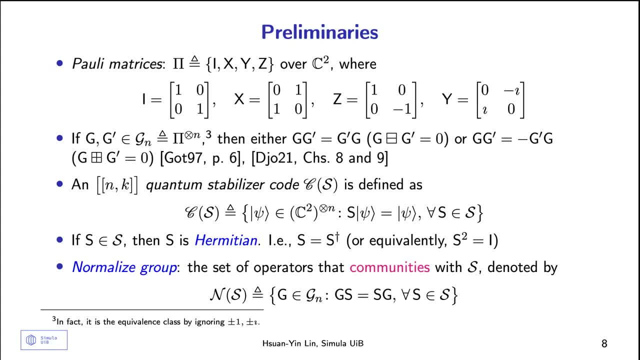 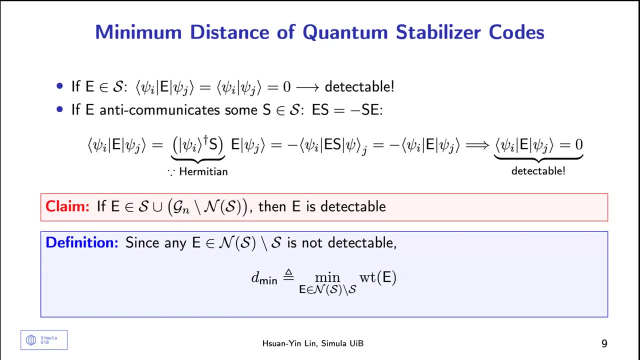 Yeah, So I hope so far it's good. I mean, I think so far it's all still classical, It's just not. we brought up the dimension to 2D and now it's matrix. Okay, Yes, So remember, we have an undetectable definition for the general quantum quantum code, but now we tailor ourself to just quantum stabilizer code. and how do they define the distance? by using the structures of quantum stabilizer code. 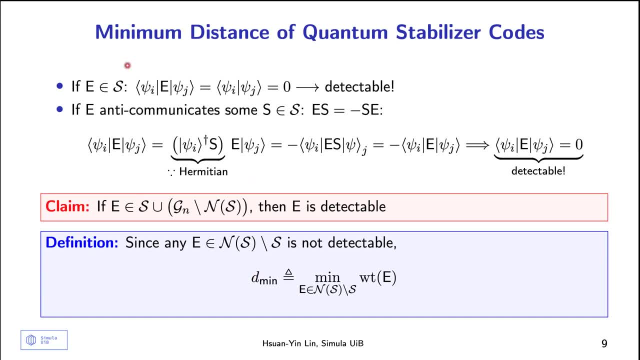 So you can prove two things. So if you have an error, error operators belong to the stabilizers And you can say: this condition which is safe by the table detectable condition, And if you have a, some LL operators is sets by listings. 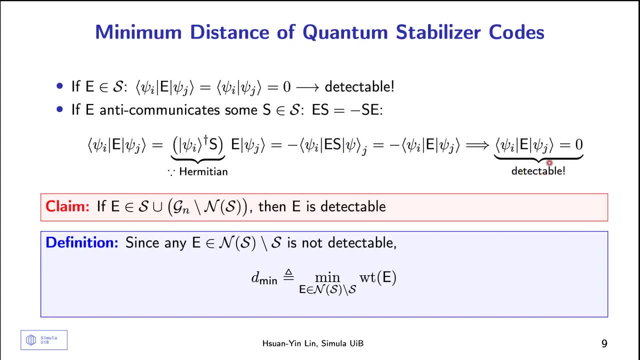 You can also show that this is detectable. So we can show that, based on the content stabilizer code, the only detectable arrows is belong to, Lee said either: stabilizers All you you set, minus the normalizers. And so how do we define a minimal distance? 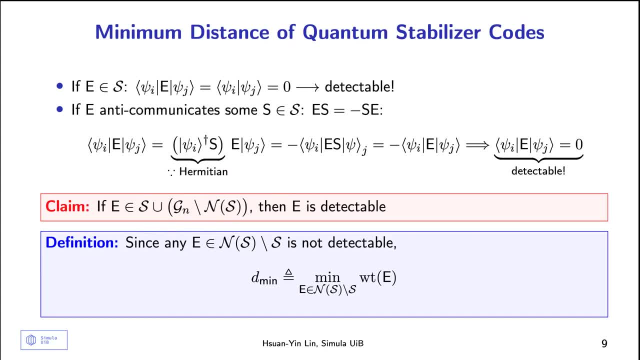 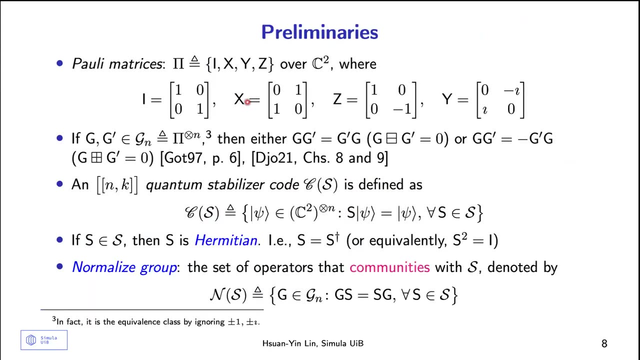 We just use the definition before we want to do the undetectable errors, so which is defined by this? So this is called a minimal distance of error. operator of this And the way to E now is more clear, right, Because the E just if you can decompose. 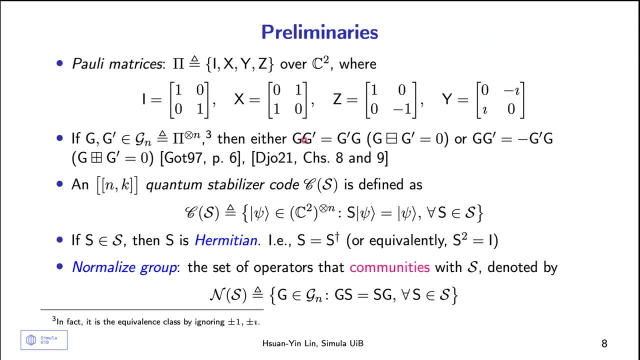 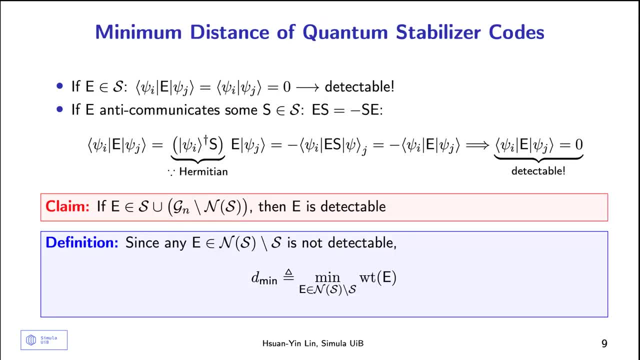 like this Pauli matrix, and they just count the number of which is non-identity. So this is how I define the minimal distance of the quantum stabilized code. Just a quick word. we have roughly five minutes left. All right, okay. 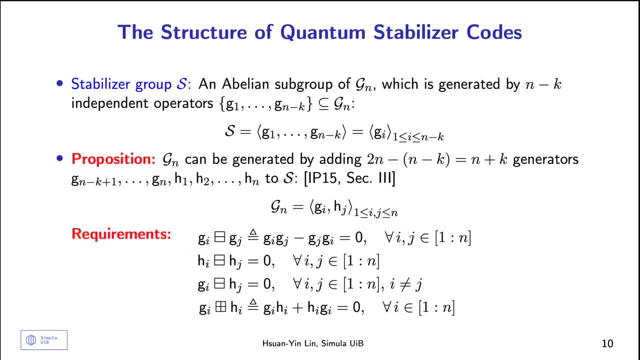 I think then, okay, I mean, let me try to do more. So, yeah, I just try to give you some take home message, not just about this fancy math. So these are the original structure of a quantum stabilized code. So these are do by matrix. 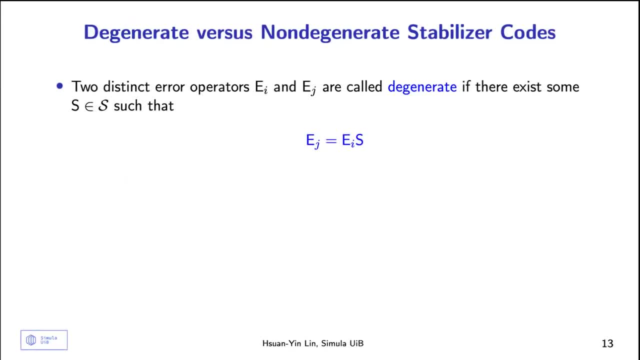 But we can do. let me just jump. We can do by classical world, by binary things, by using something called symplectic code, symplectic codes. This is what's proposed by Cardiff and Rance. I didn't show and I don't remember what's the last S, but 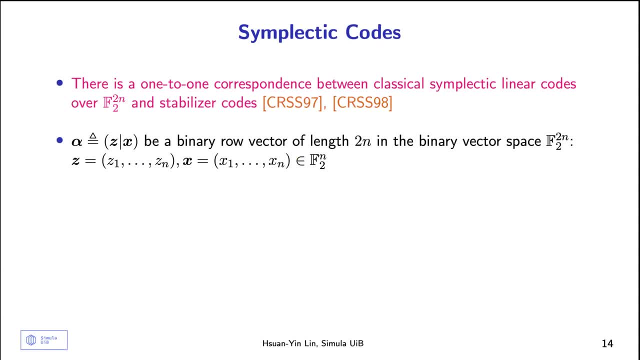 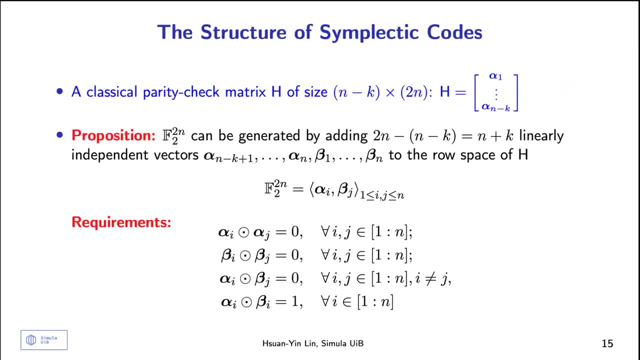 Anyway. so we can describe such quantum code by just binary vectors actually, And the forget list. so this is the main message I want to say. So forget how quantum matches you do? You just pick length two times n, binary vectors like this: 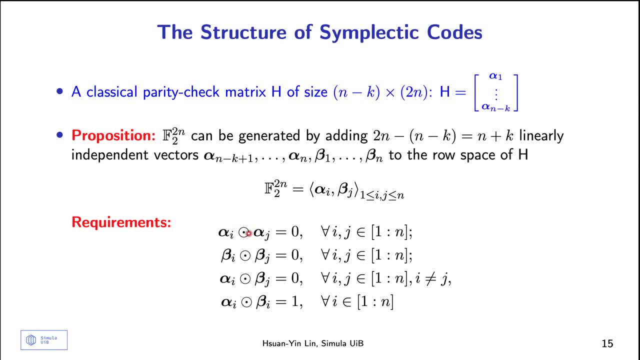 And these vectors satisfy this condition. This is called symplectic inner product And you need to do some symplectic version inner product, But it's still a complex space within where defined between inner products, So it's still a linear algebra. 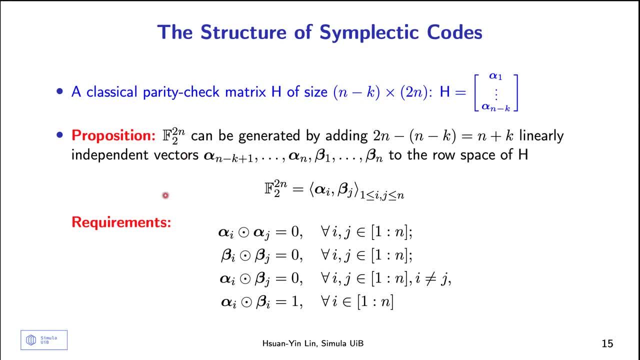 It's just an operation you need to change And then you can find those basis to satisfy these things. Then you actually are done. So you already find a code in classical world, but still you can tell what happened in the quantum stabilized code. 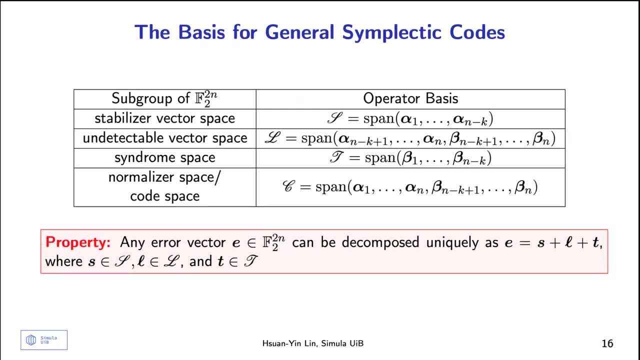 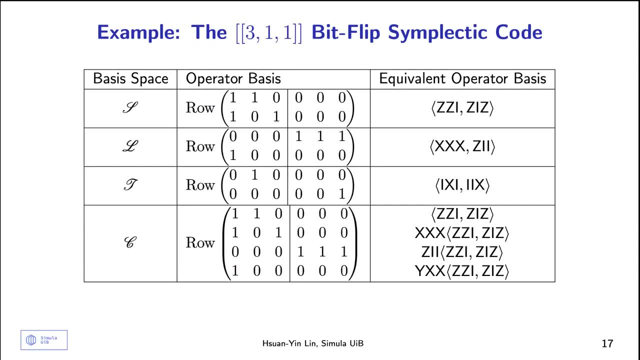 So this is the main message I want to say, And I did try to get some example, You can see here, And yeah, we don't have too much time. And the other thing I want to, actually want to say in the abstract, is the degenerated 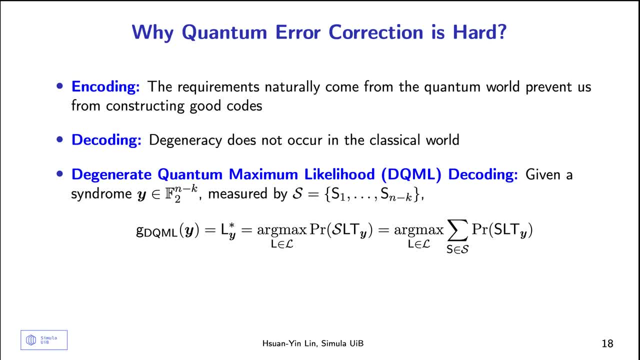 So the one thing I want to emphasize: in quantum world the degeneracy does not occur in the classical world And it's because of the stabilized definition. And then it changes the way of decoding of errors And in such a lot it would be rewrite to like these things: 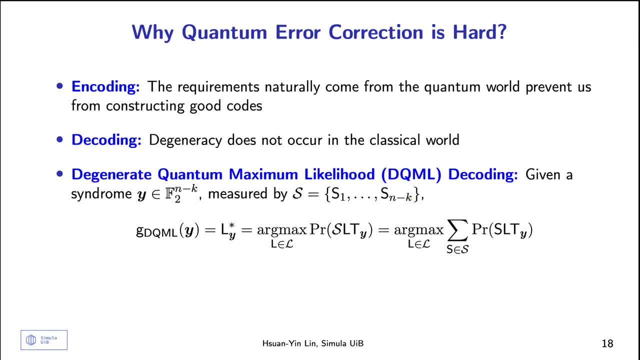 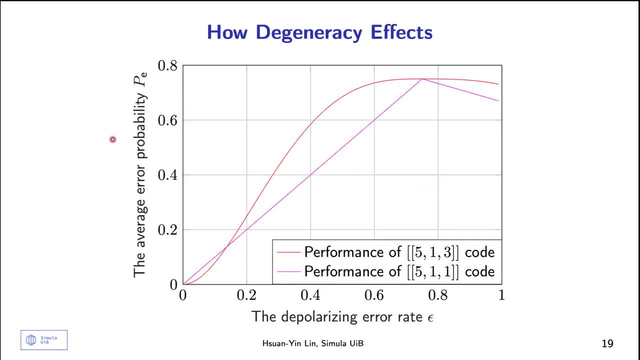 But again, this is just math but I just want to show you some. actually this is related to some research I'm doing now. So how actually degenerate can affect the quantum code we pick? is that in classical thing we would believe? 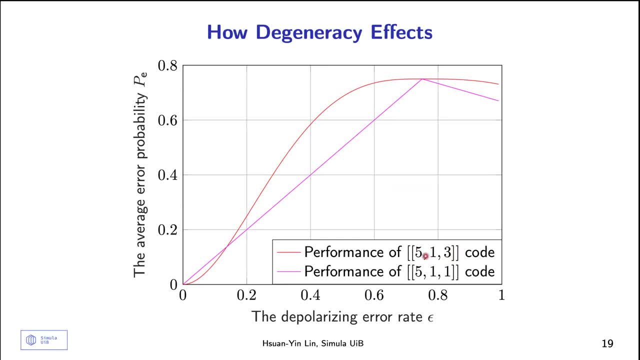 okay, the distance three code in the five one- this means five qubits and one dimension- is better than the. this is just the smaller distance codes. But if you really compute the average error probability by this degeneracy you will see that actually this code is only good. 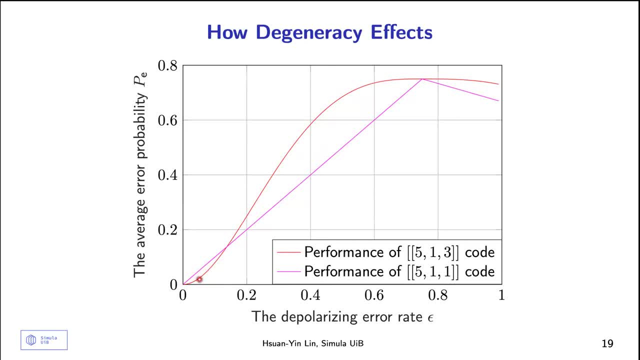 in this very certain range And this actually happened a lot in five people. it's very hard to find good quantum code because it's hard to design and it's hard to predict And for most of the time actually they just use repetition code. 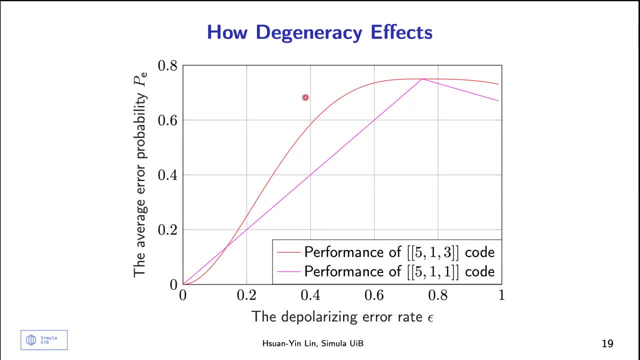 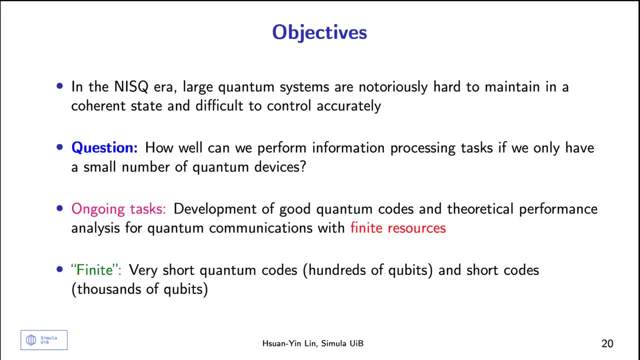 Small distance code is still good, So this is the one message I want to share here. So, yeah, this is just the yeah final slide. So I mean our goal now, what we are doing with our PhD and our lab, is that we want to develop a good quantum code.